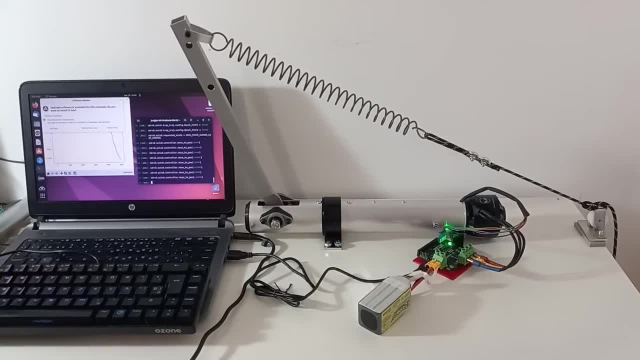 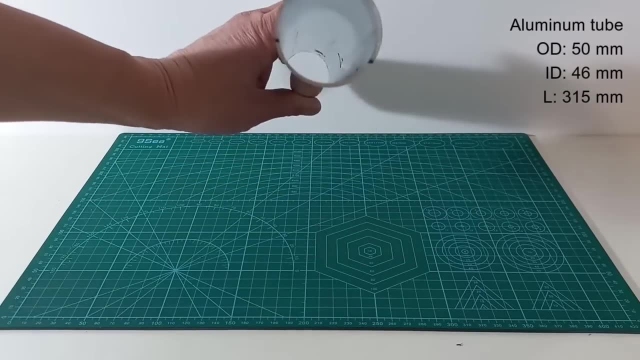 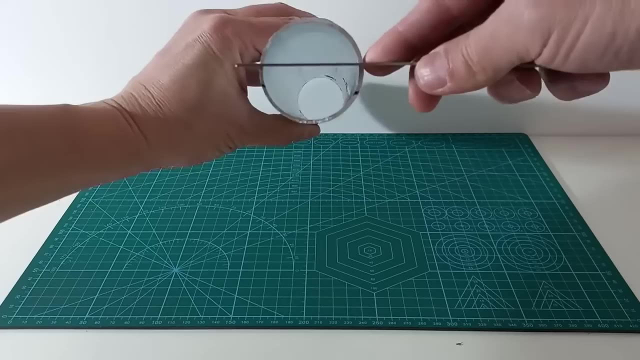 At the end of the video. we will test it and see how powerful it is. We will start from a 50 millimeter aluminum tube in which we will open a window and drill two holes for the joint shaft. The holes for the shaft will not be in a diameter of the tube, but in a lower position. 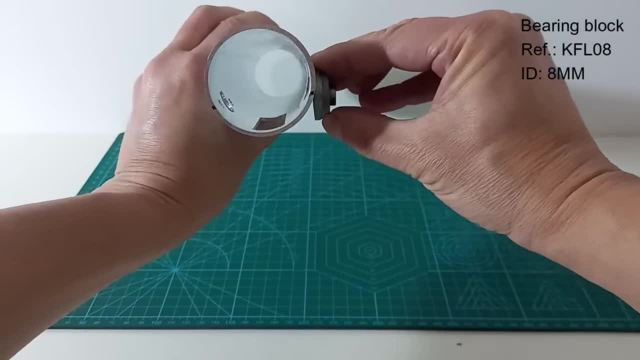 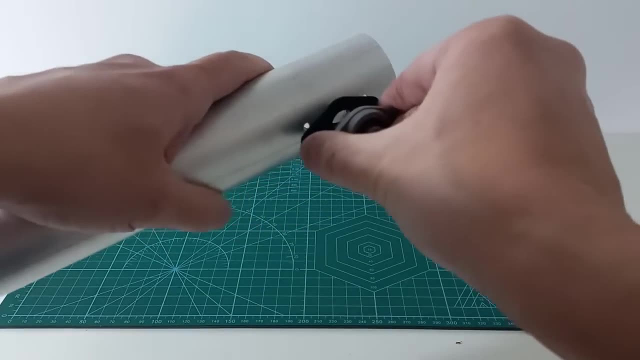 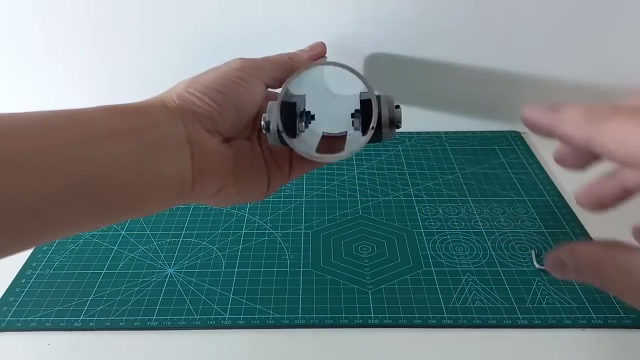 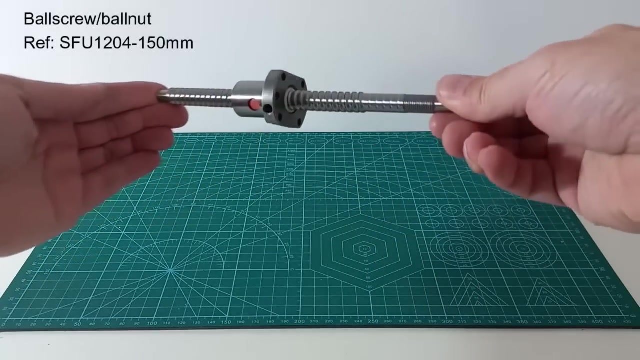 We will install two bearing blocks to hold the shaft. Before that, we need to adapt the curvature of the tube with a 3D printed part. Similar adapters are used in the inner part. The ball screw and ball nut model is commonly used in 3D printers. 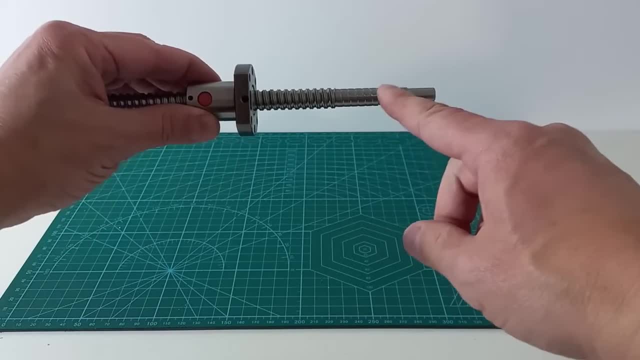 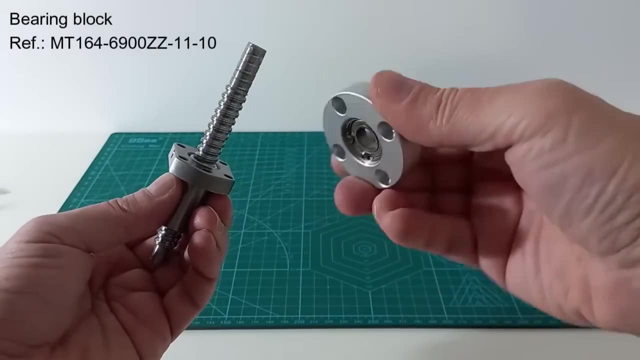 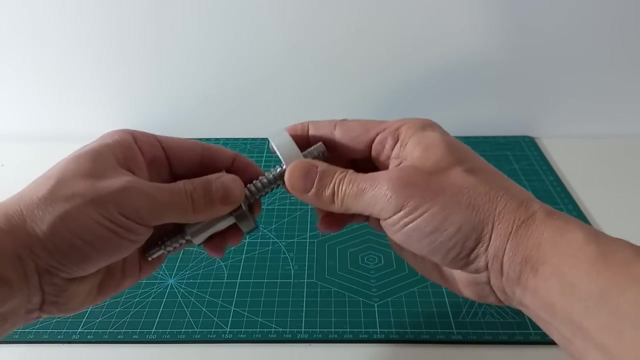 We will remove this threaded part to make it shorter. We will use another bearing block for holding this side of the ball screw, but before installing it we will open a groove for the encoder cables. Now we can install the bearing block which will take radial loads. 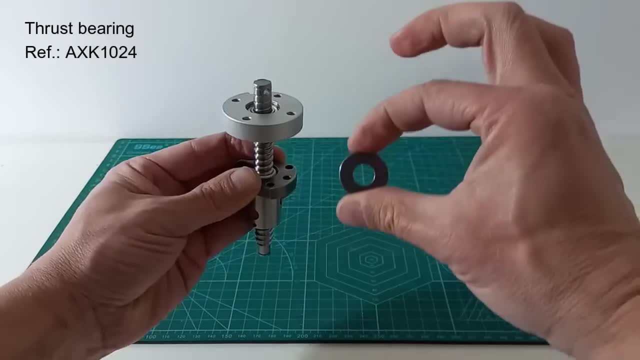 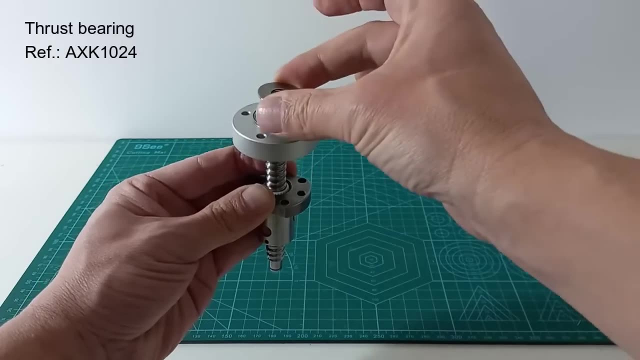 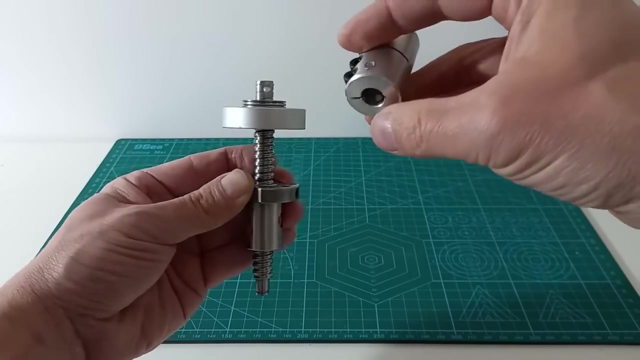 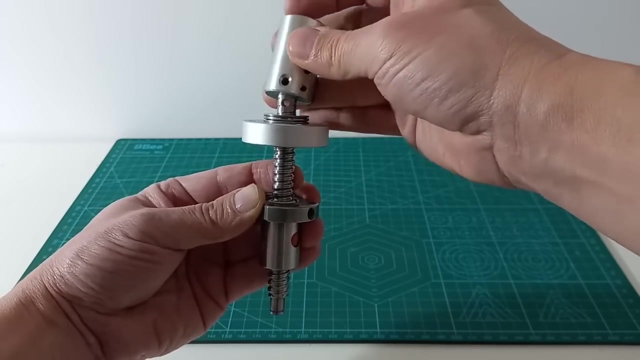 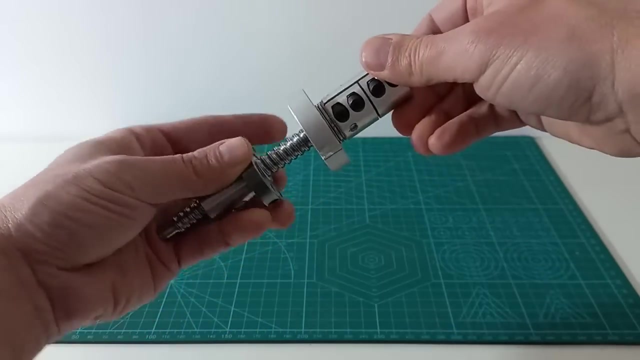 We will add a thrust bearing, since forces of the ball screw will be mainly axial. A 10 millimeter coupler will join the ball screw and the motor shaft. We have drilled the ball screw and the coupler to install a pin that will prevent motion between them. 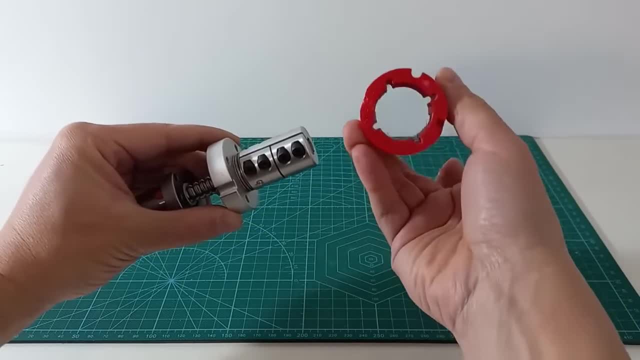 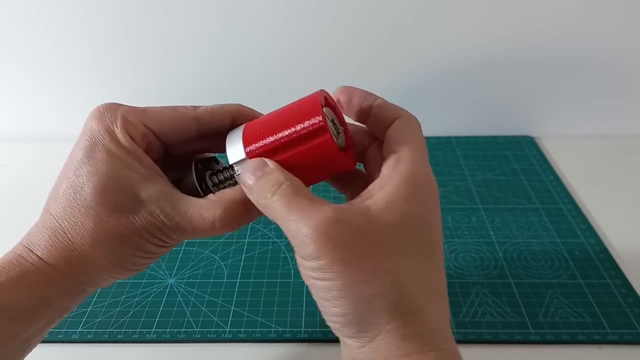 A 3D printed spacer will hold everything centered in the tube. None of the 3D printed parts are structural Testing. the parsleymayim motor will respond with possibility of moving the output. We can also add a slide system by pressing both these pedals. 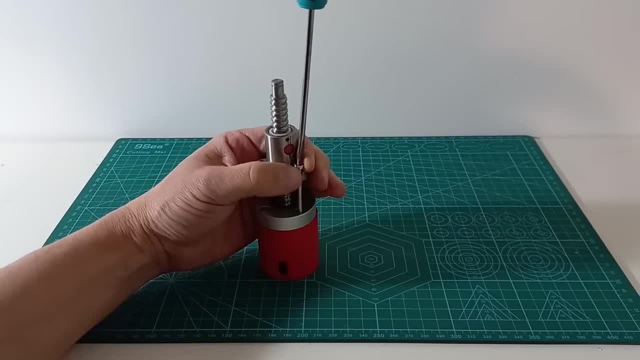 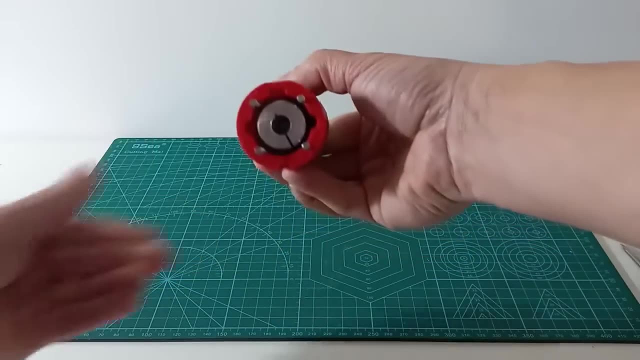 The slam feature is a very dwellable product, so we will click the designed 하나 feedback. Using the 3D printed spacer, we blast the material that we need before we start judicial 안 использовать For the following structure: we will useJulian and the Law EMF model with the spring system. 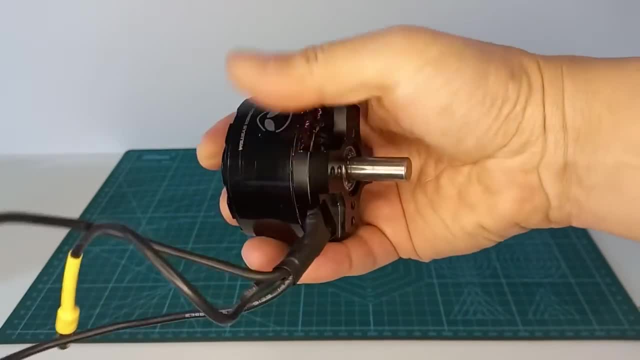 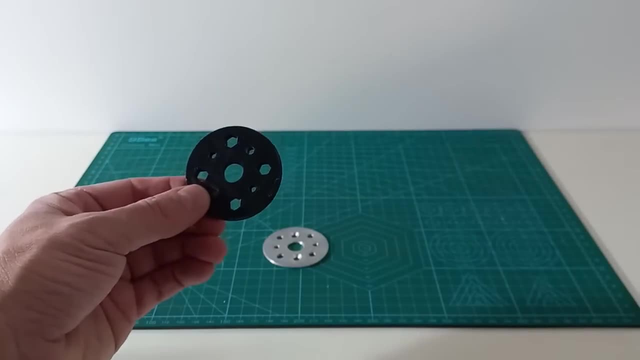 The brushless motor model is commonly used in electric skateboards and has a very high torque, 6 newton meters. A laser-cut aluminum disc will adapt the motor to the axles and manageret Dublin motor to the post crew set. A 3d printed disc is used to hold some nuts. 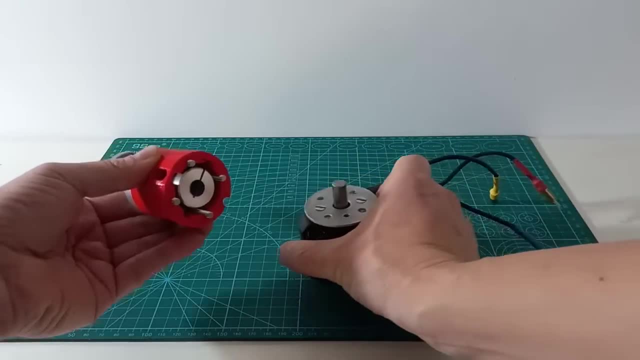 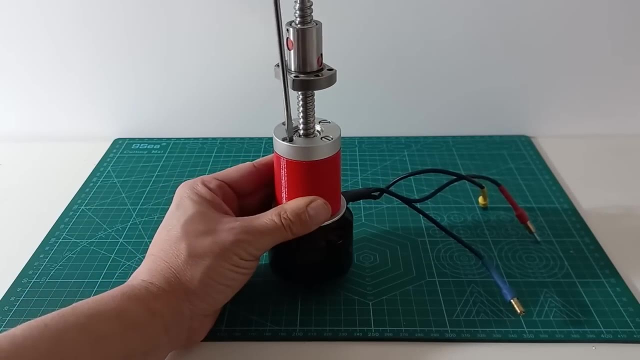 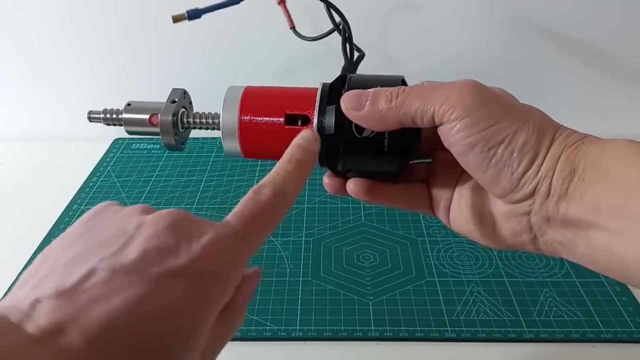 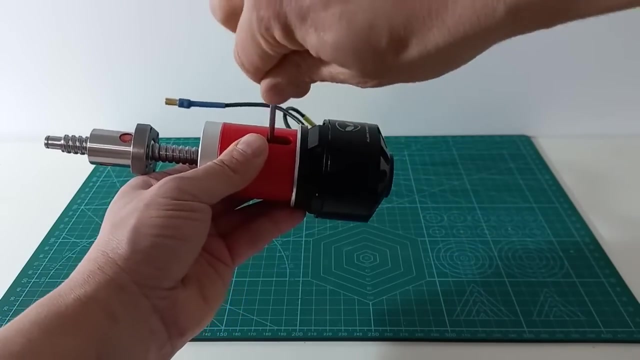 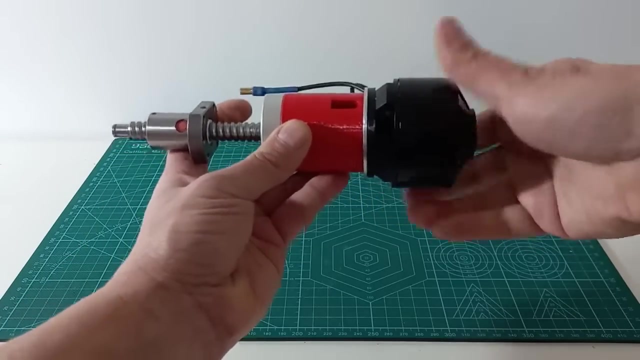 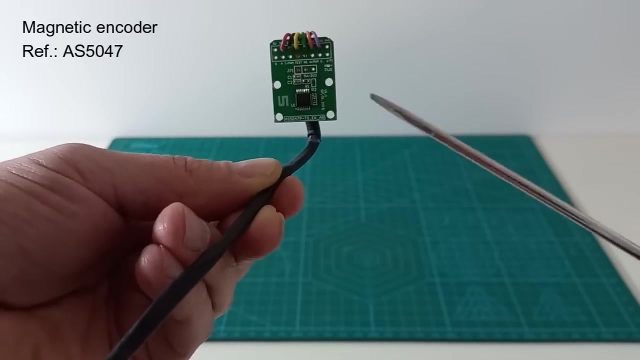 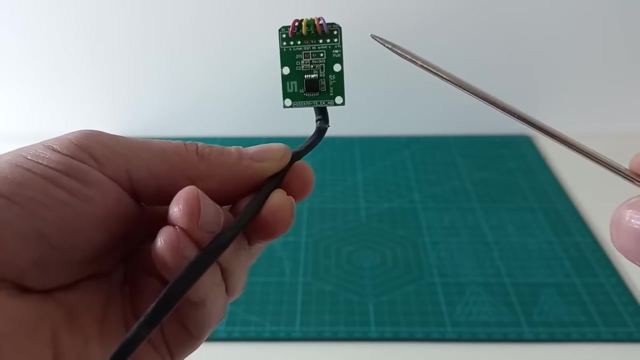 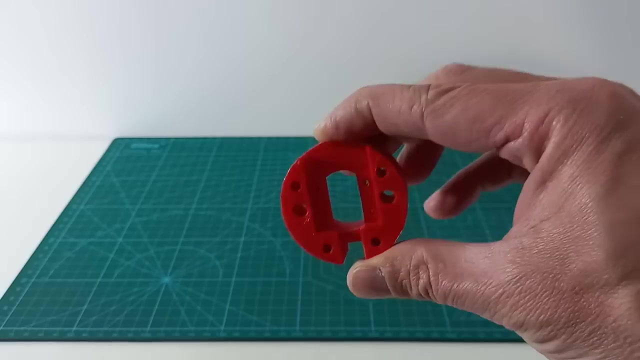 Now we can assemble the motor set. The shaft coupler can be tightened through a window. Now we will install the magnetic encoder. Here you can see the magnetic set. I have already soldered the wires to connect it to the controller. A 3d printed part will link the encoder to the ball bearing. 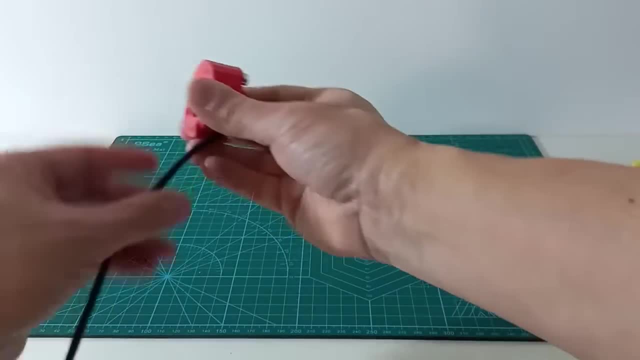 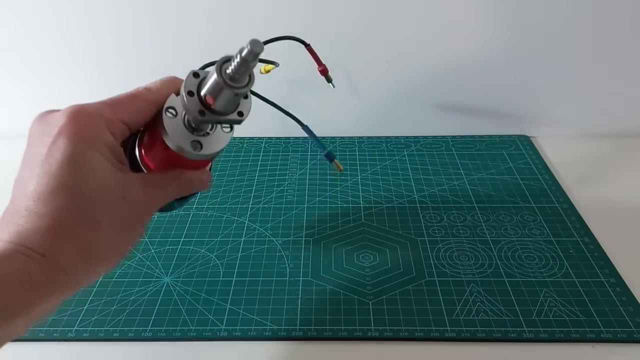 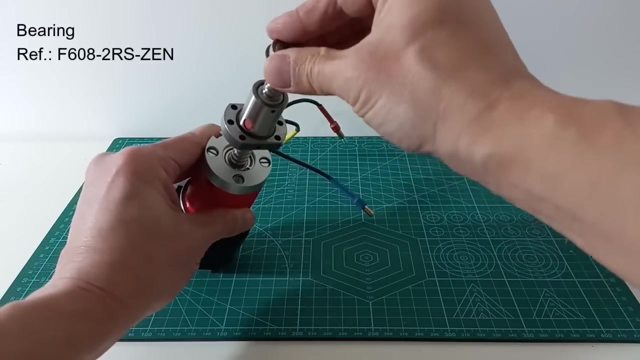 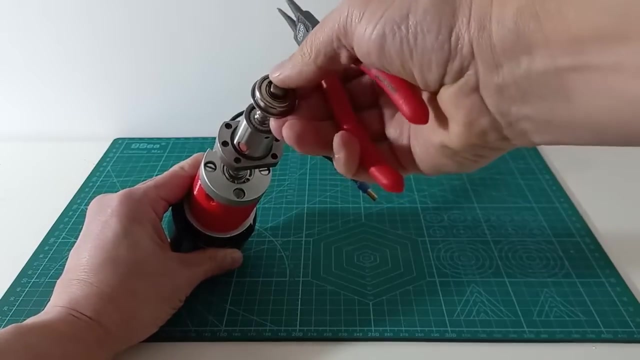 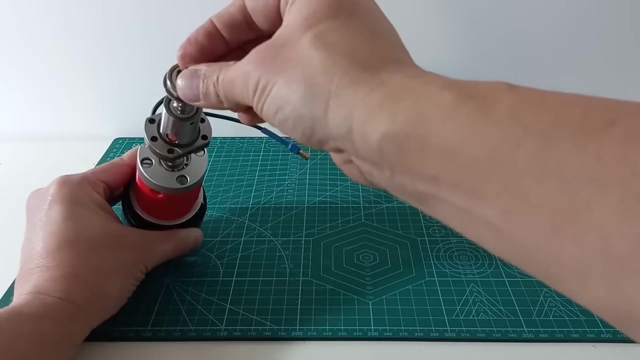 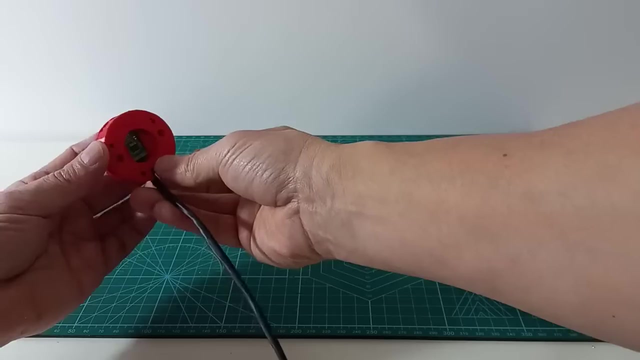 A cover is used to protect the electronics. In this side you can see the magnetic sensor. Now we'll install another ball bearing with an external clip And the magnet for the encoder is glued to the ball screw. The distance between the magnet and the encoder must be less than 3 millimeters. 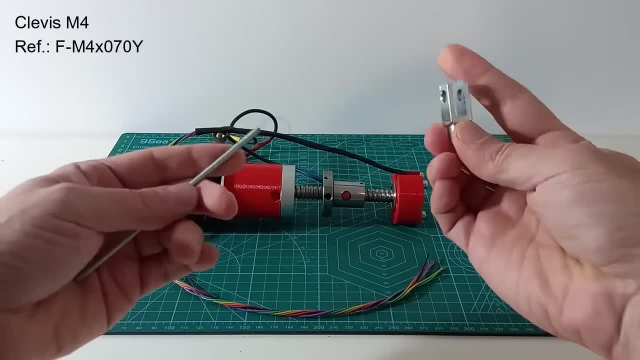 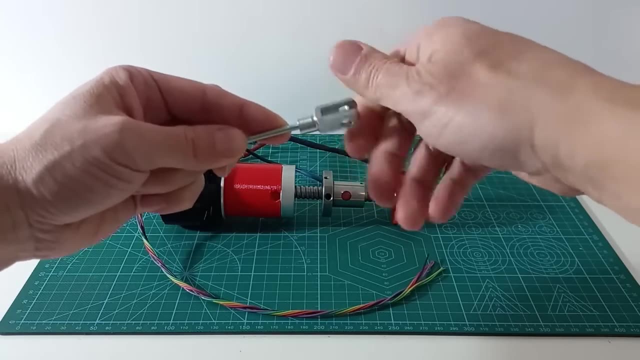 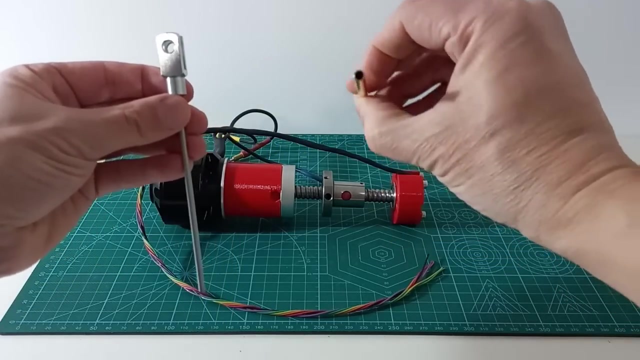 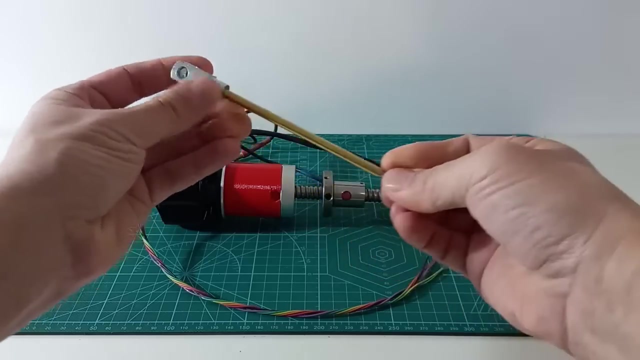 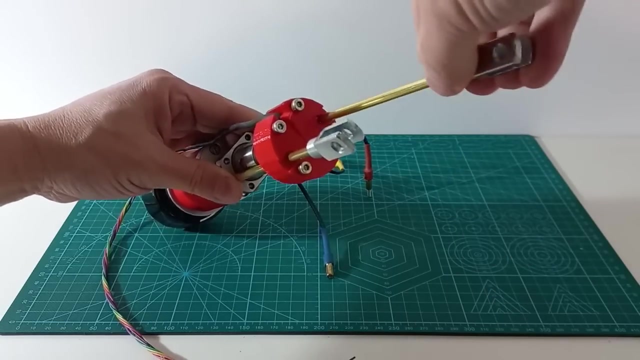 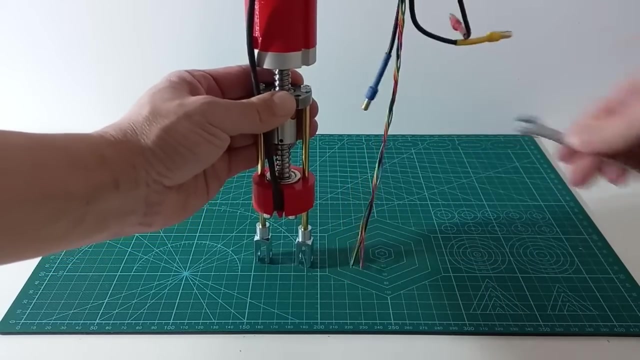 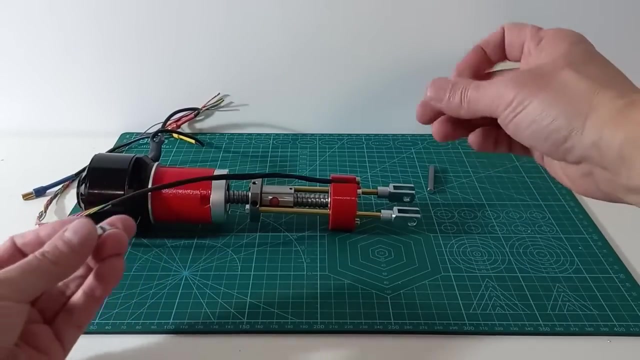 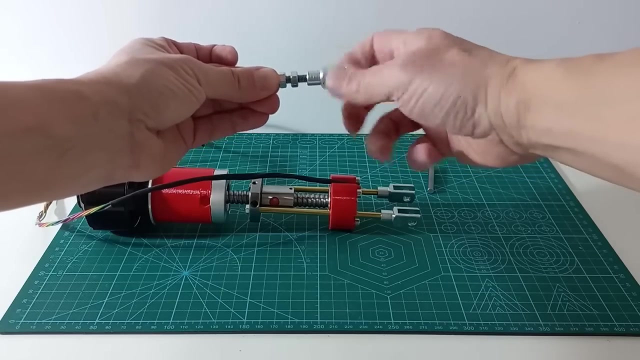 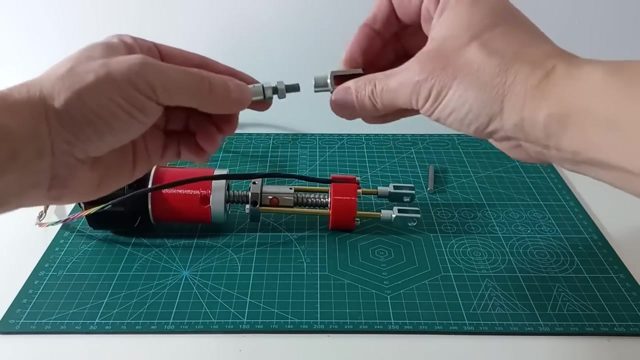 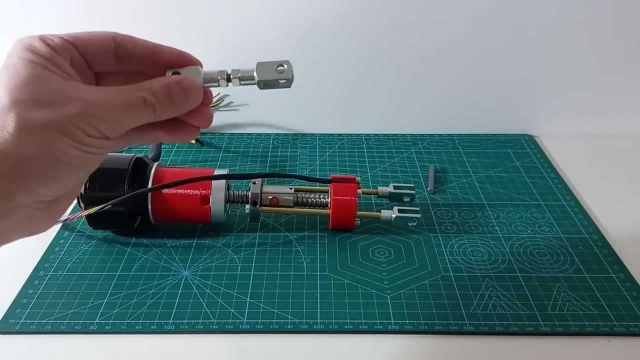 Now we will build the output rods. A connecting rod is built in a similar way. A connecting rod is built in a similar way. A connecting rod is built in a similar way. A ball bearing is used to allow the rods slide along the tube. 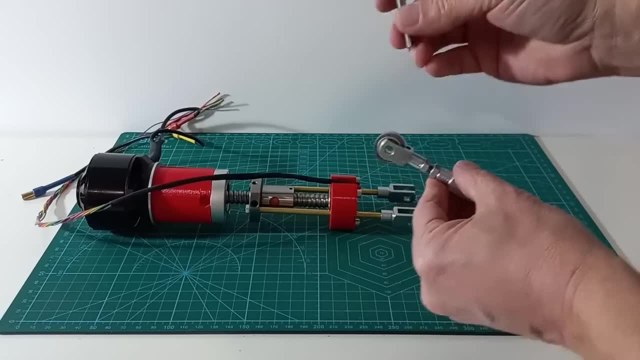 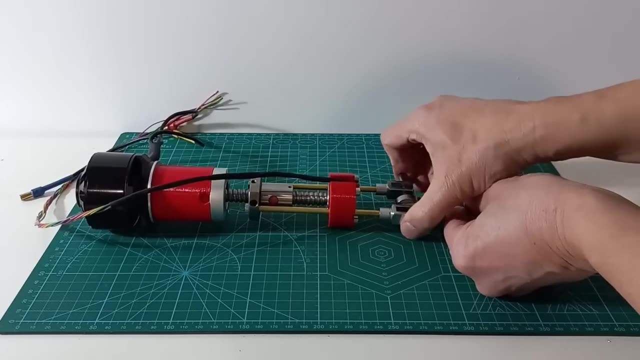 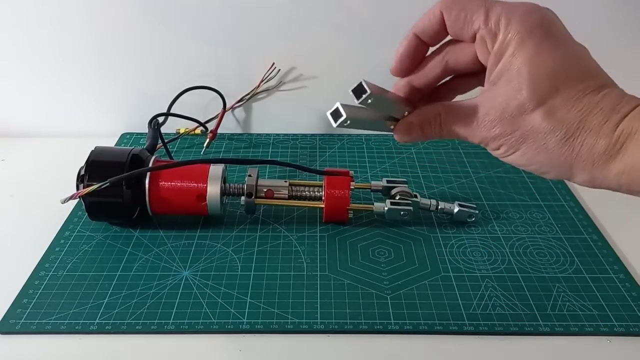 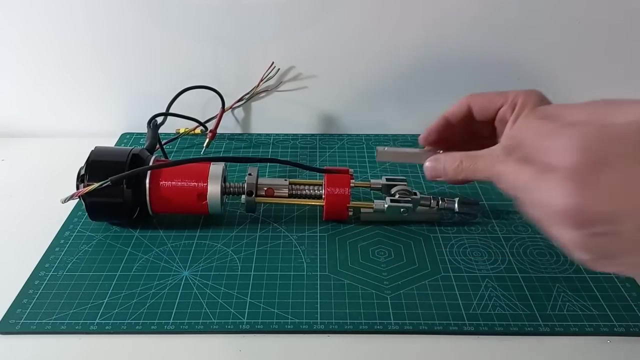 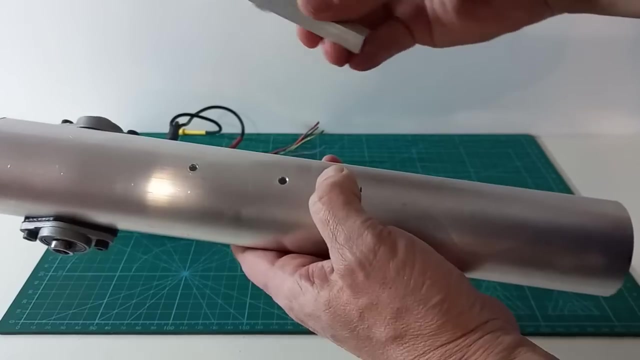 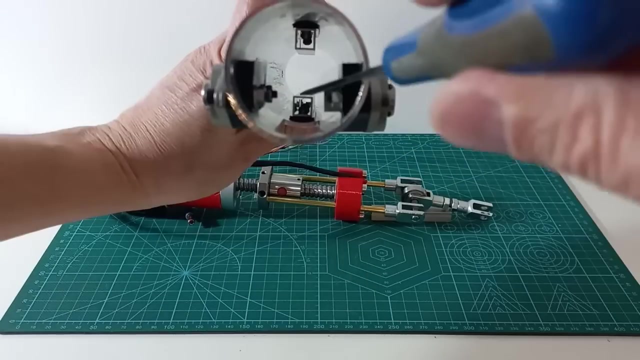 The connecting rod is joined to the output rods with a pin. The connecting rod is installed to the mechanism of the pull nut. Next you will set the rod Savior. The ball bearing will slide between two aluminum parts. These parts are fixed to the tube with rivets. 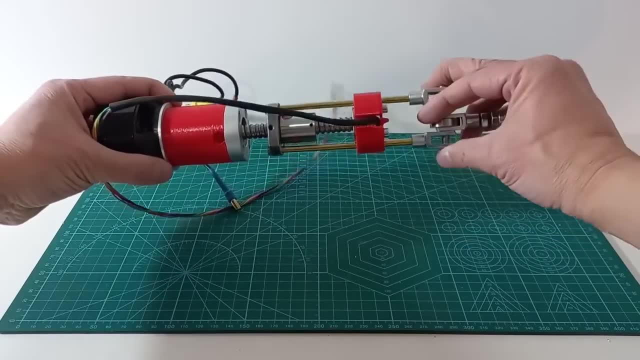 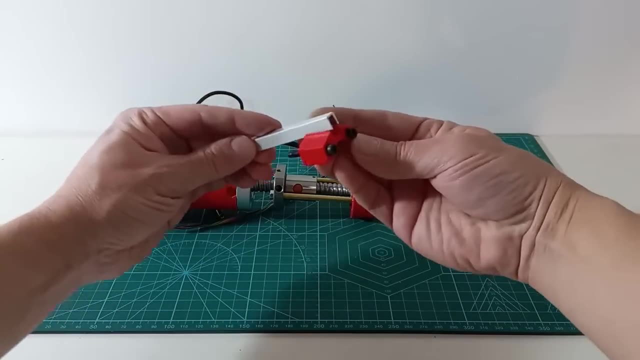 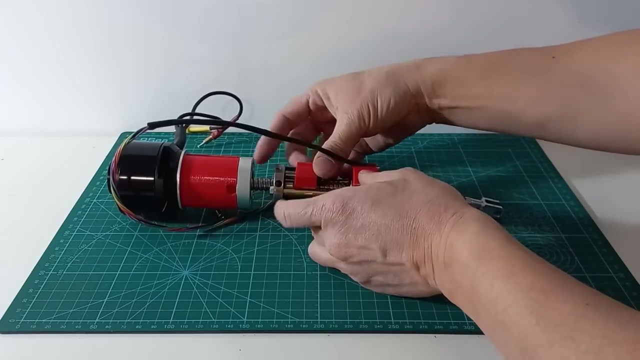 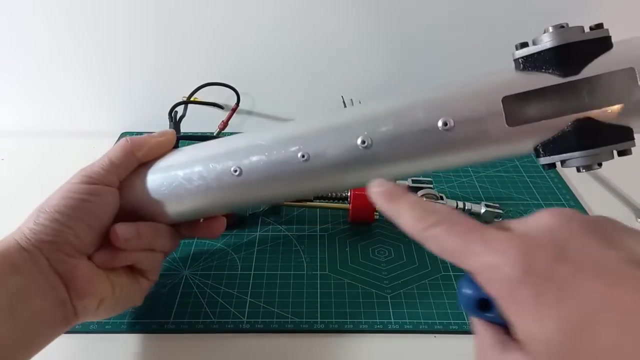 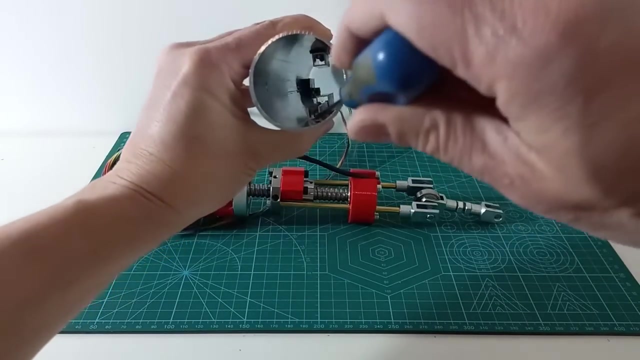 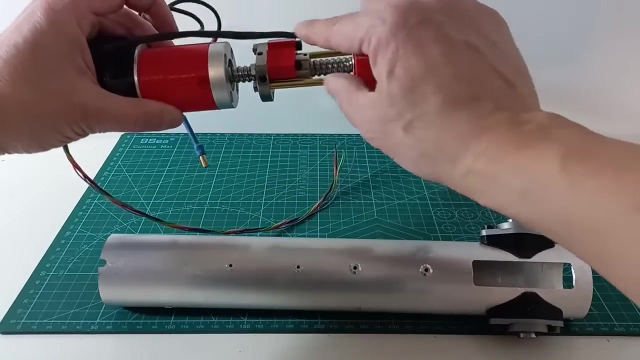 Now we must prevent the ball nut from rotating. We will do it with a 3D printed part that will slide along an aluminum profile. The aluminum profile is also riveted to the tube. It will also be used to guide the encoder cable. 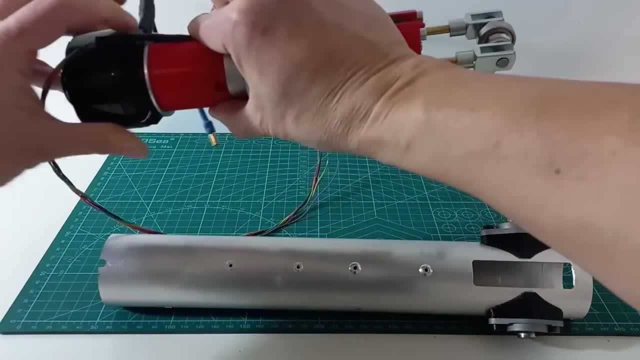 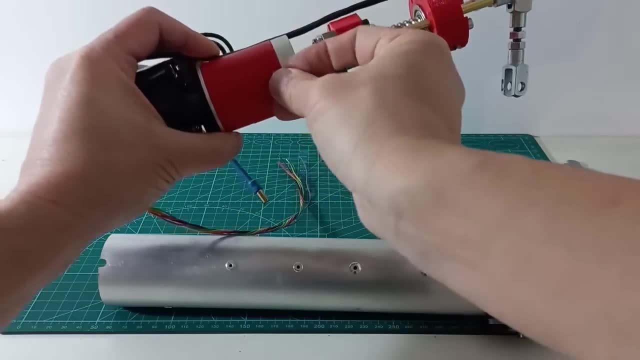 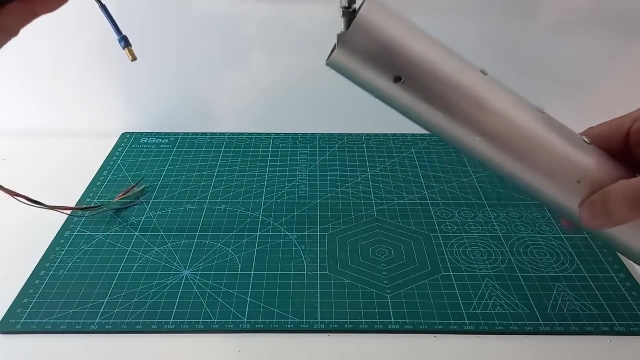 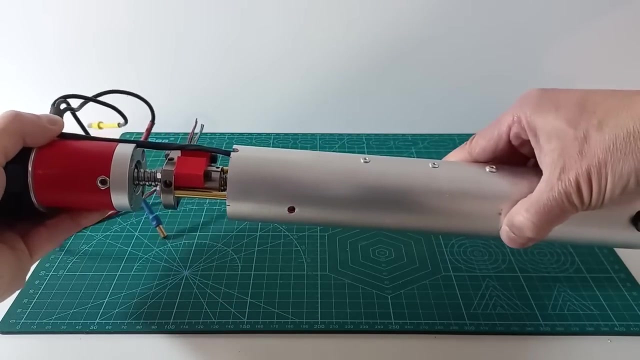 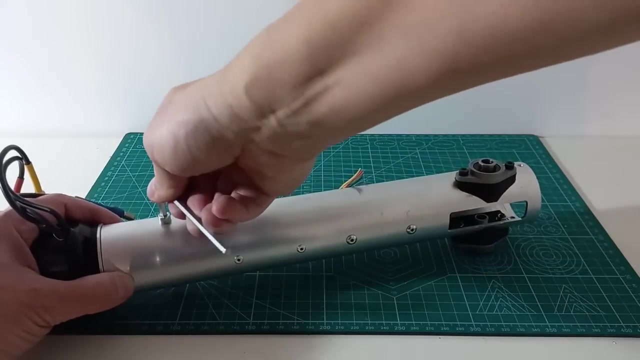 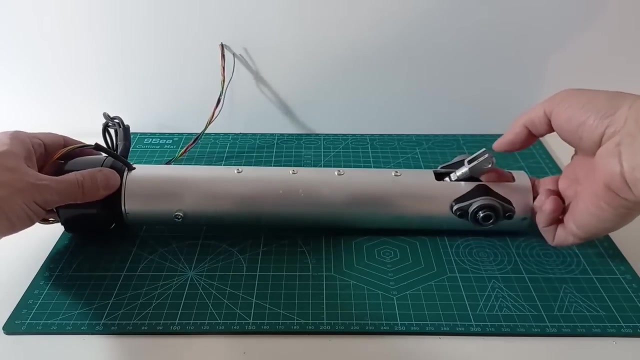 Now we can remove the ball nut. We insert some nuts for fixing the hole set to the tube and we assemble the hole set. Now we will connect the crank to the output rod and to the joint shaft. The crank is a laser-cut steel part. 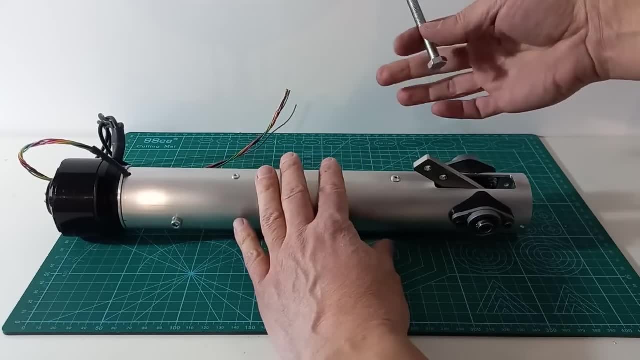 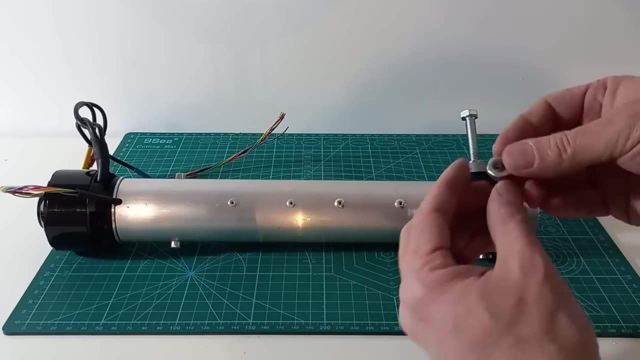 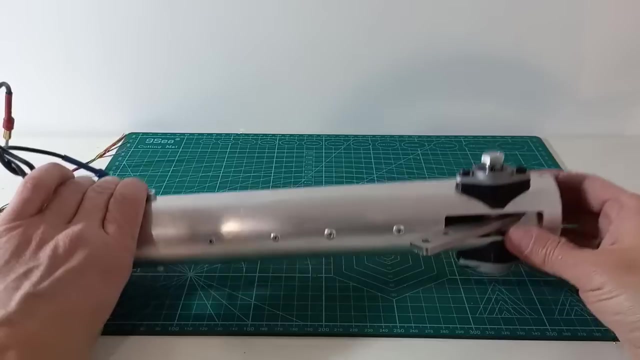 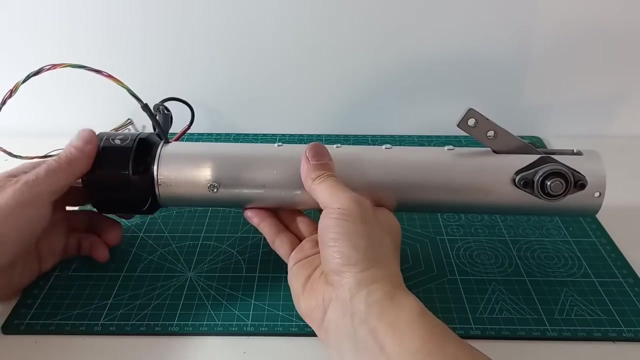 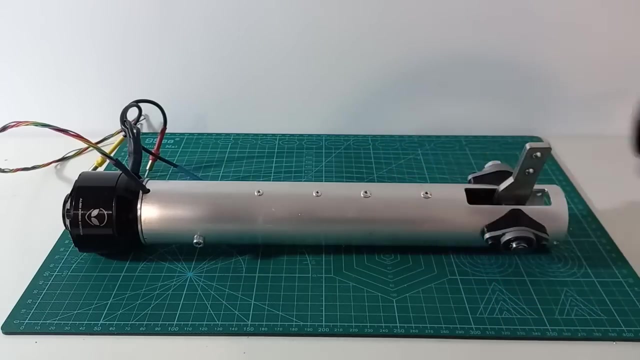 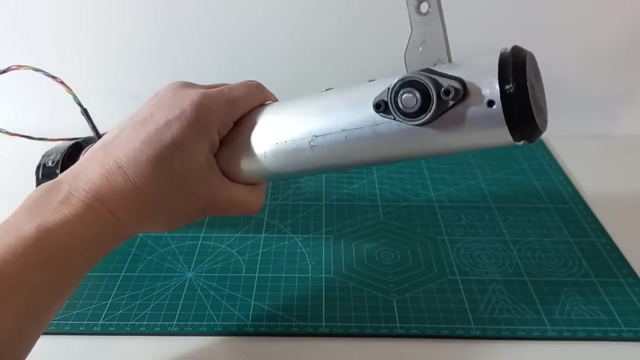 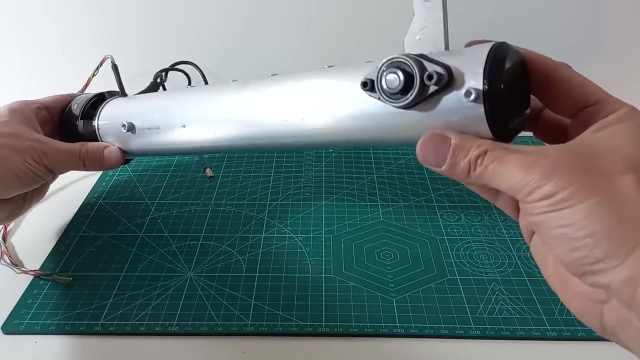 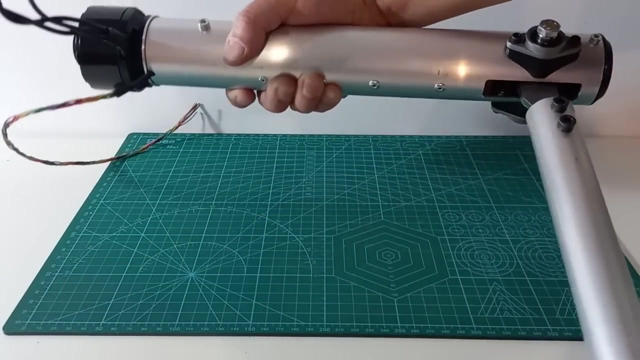 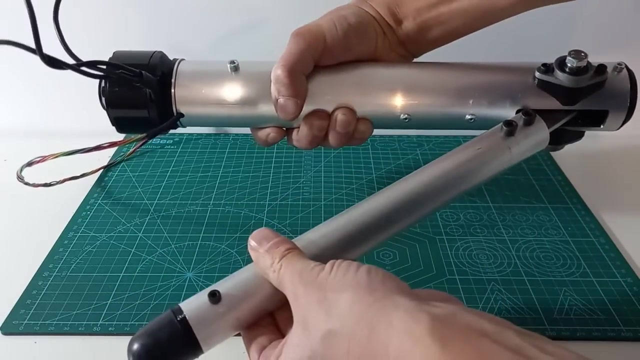 The joint shaft is an 8mm bolt. We will use two nuts to fix the crank. Finally, we put a cover to close the tube. Here you can see the final result, with a link resembling a robotic leg. The actuator is easily back-draidable, as you can see.